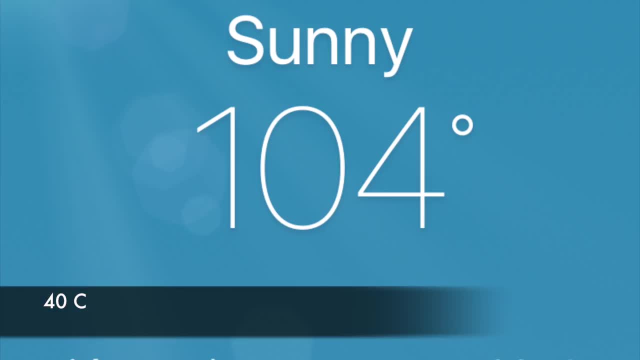 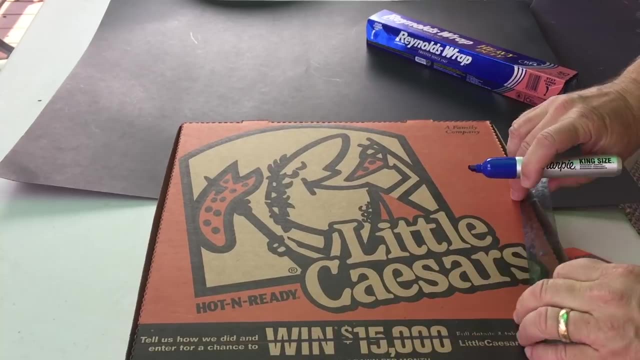 which I have, as today is 104 degrees in Northern California, So we're going to do the solar oven To set this up. I'm going to do two different experiments. The first one's with a pizza box and the second one is a regular box. So I'm going to outline the pizza box about an inch away from 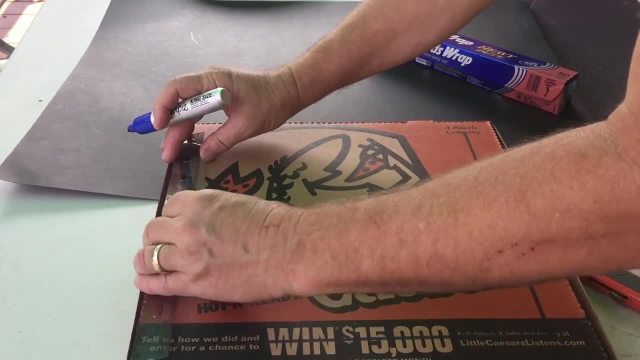 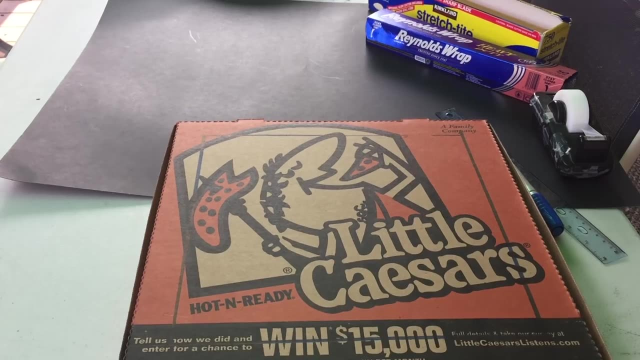 all the corners, And so you do all four of those corners like this, and then you're going to take a box cutter and cut that out. So now we have all the lines traced out, We're going to use a box cutter and be very careful, A box cutter can cut you very badly. so have adult supervision. 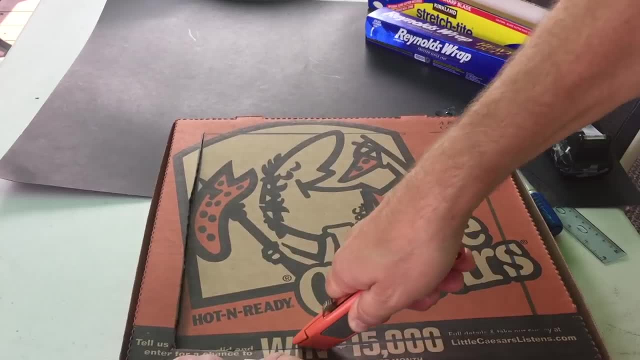 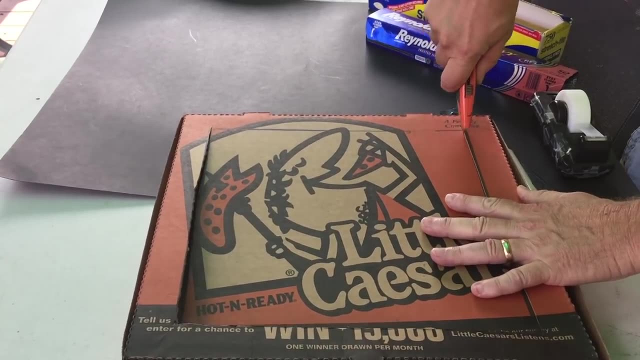 And we're going to cut out three sides. So the front of the box it pivots up what I'm cutting two sides, not cutting the back part of it. You just want to stop about an inch in there and then you can flip it up just like this, So you don't cut all four sides, but if you do, 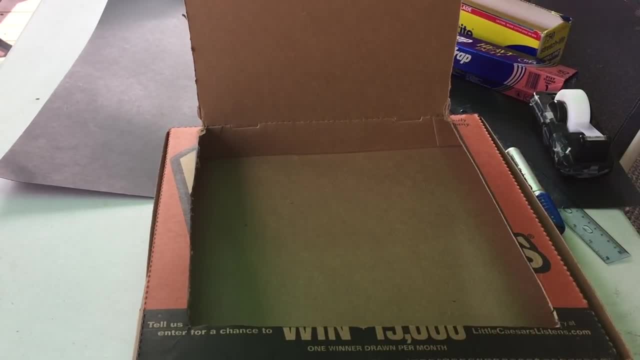 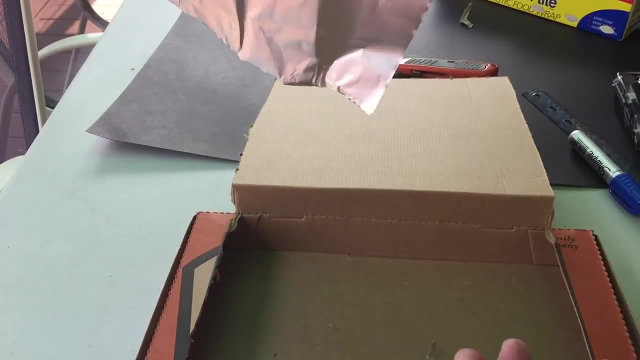 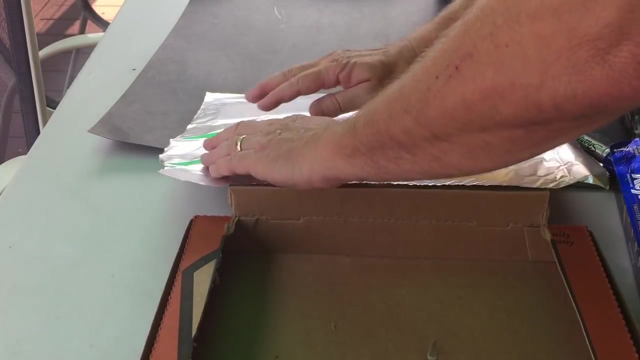 you can just tape it on, Anyway. so there it is. That flips up just like that. And then now we're going to take some aluminum foil and we're going to foil the piece that we just flipped up. So go ahead and pull out a piece of foil and you lay it on the back, just a little bit bigger than 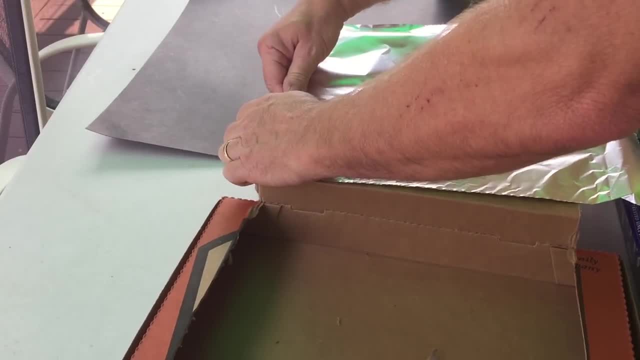 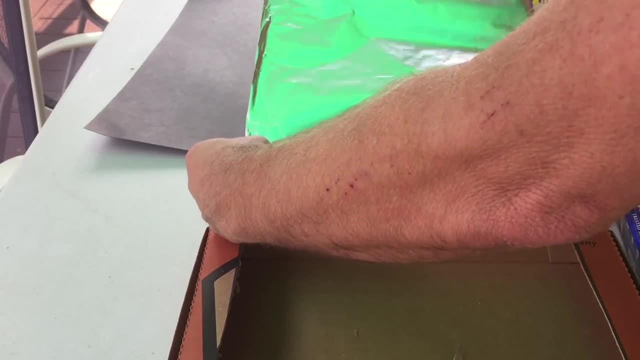 the flipped up piece itself. You're going to fold it over and then we're going to use scotch tape or any kind of tape to tape it to the top part of the box, which I'll show you in just a second. So now I got the top. 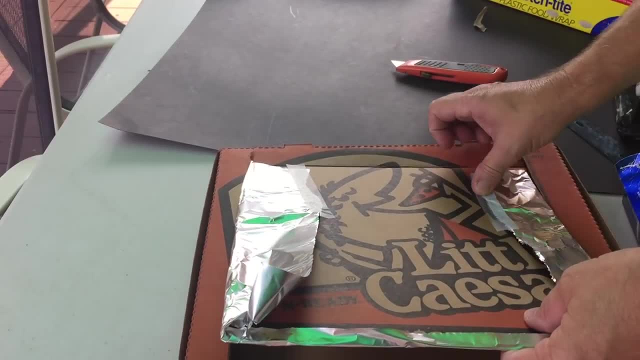 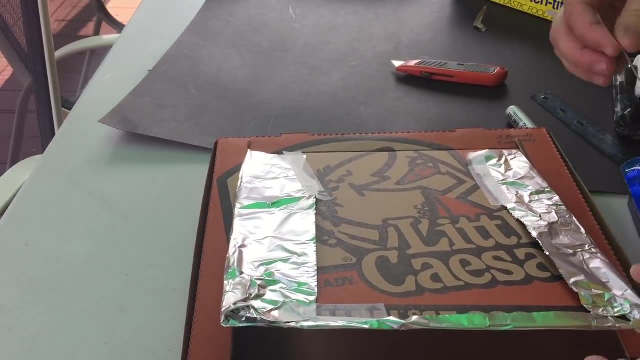 part of the piece that we cut out, and now I'm just taping it so it stays on securely. It's better to have the tape on the outside than inside the oven because of any toxic fumes that could come off the tape, which shouldn't really, but this way we're more safe because the tape is always going to. 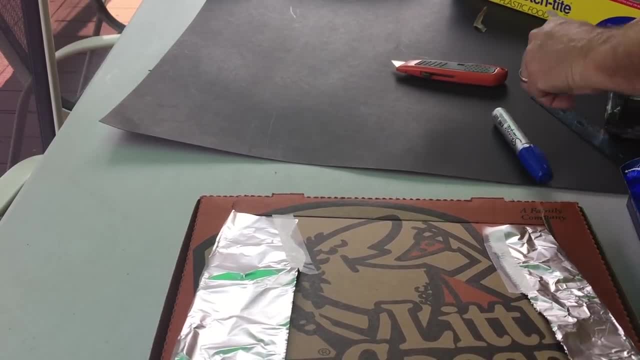 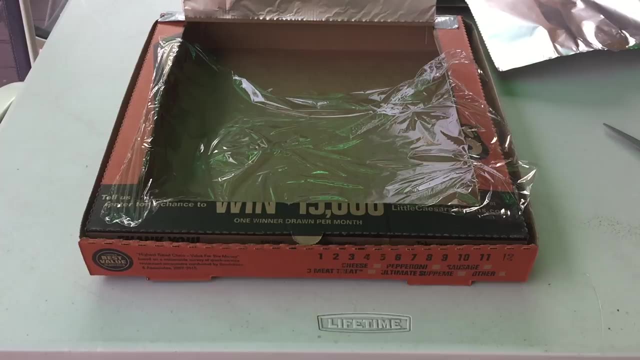 go to the outside of the oven, And so I'm going to tape that all the way so it doesn't rip off. And then, once I get that done, we are set on that piece of it right here, And that's the part that the sun's 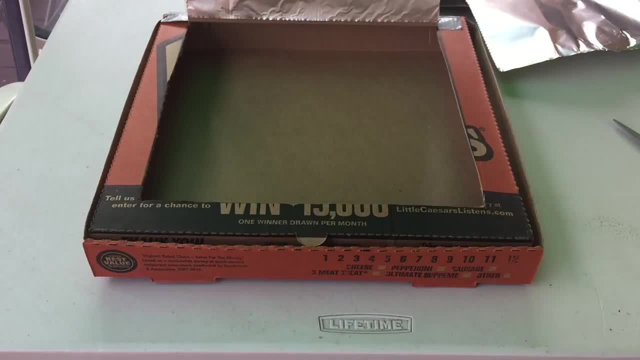 going to see. So now we're going to make like a glass window. So we're using plastic wrap, saran wrap, and we're going to go over the top of it and we're going to tape it down. You want this. 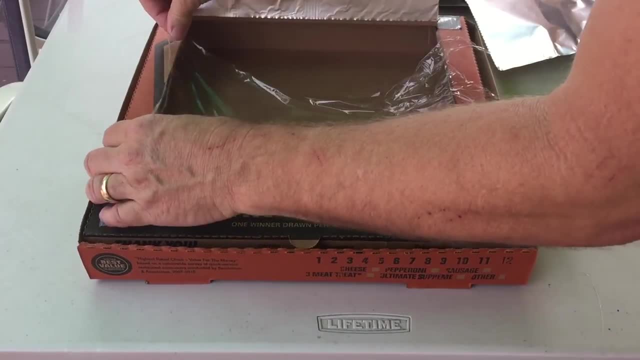 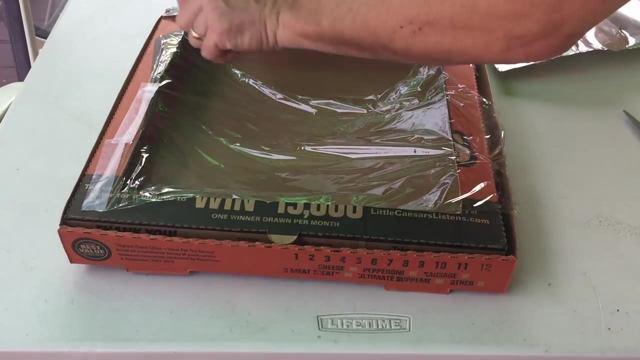 stretched out nice and tight. Now my piece wouldn't cover the whole box, So A I could have measured the box and just cut the piece If I was really smart ahead of time and had it fit this piece. but you can use two different pieces. that 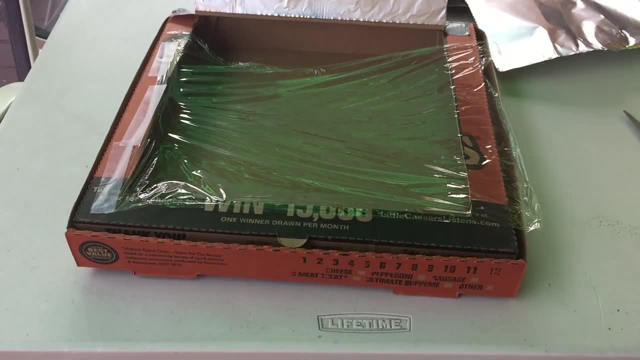 I'm going to show you here, And so you make sure you pull that tight, And then what we're going to do is tape the sides, and then we're going to come back and tape the bottom, and then we'll add a second piece. 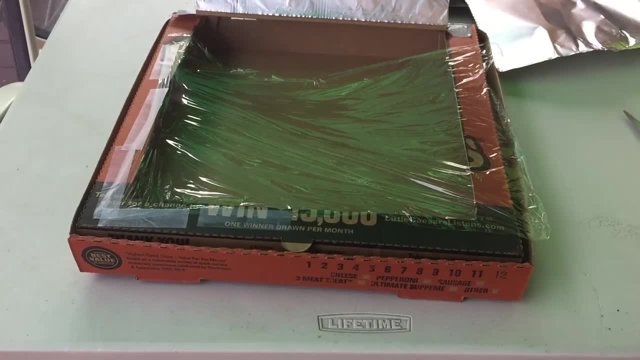 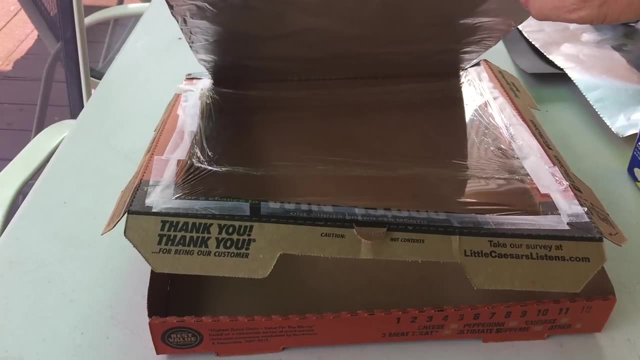 in just a second. So I ended up finishing the taping up a little fast here, and then I taped all the sides and then I'm going to add a second piece. So now I've got a second piece on there too, And now I flip it. 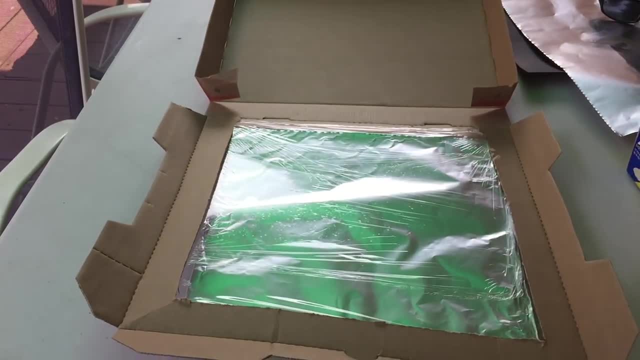 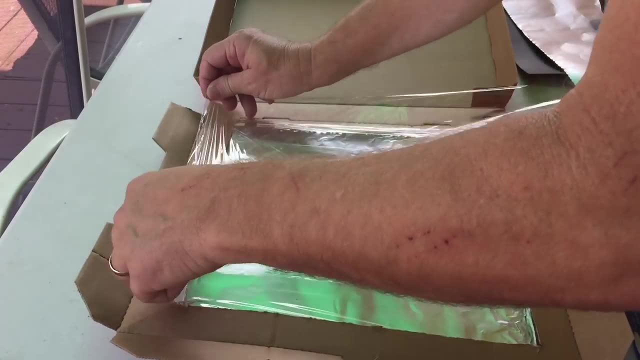 upside down, and I'm going to put a second piece of plastic or saran wrap on the bottom part, because you do not want any air getting in or out, And so this will be helpful. This is optional, You don't have to do this, but I find it. 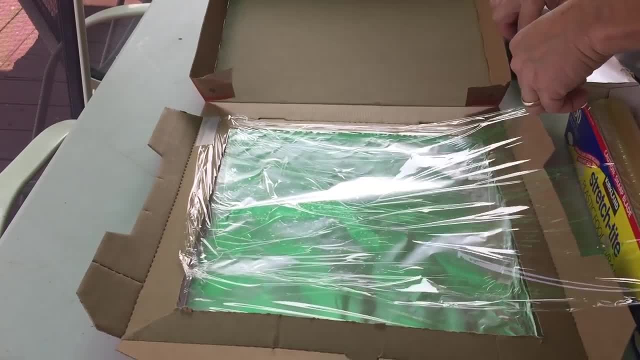 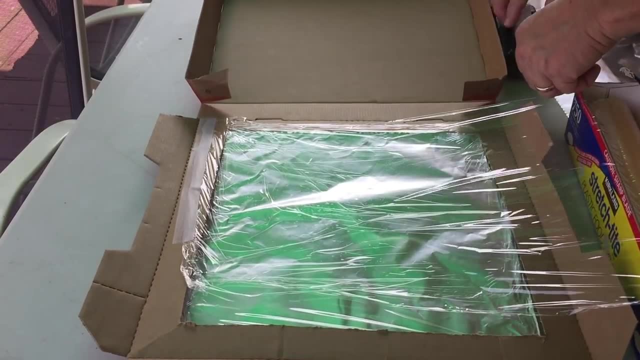 seemed. it works pretty good for me and it doesn't take up all the do So same thing. get your saran wrap, put it in. You're going to use two pieces again. Tape it all the way down, cut it out so it fits in, and I will speed it up and 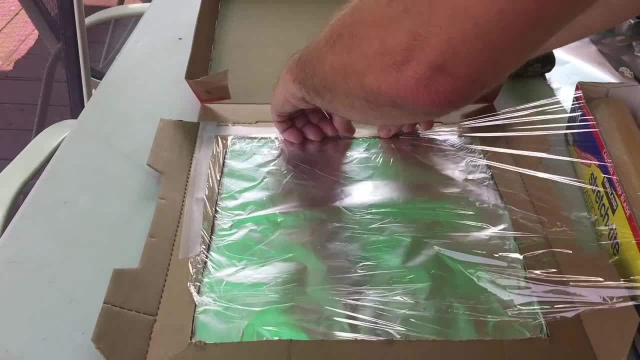 we'll get to the point where I'm going to put it in. So I'm going to put it in, and I'm going to put it in and I'm going to finish. We'll put it in fast motion here and we will get that piece done and cut it off and then tape this piece. 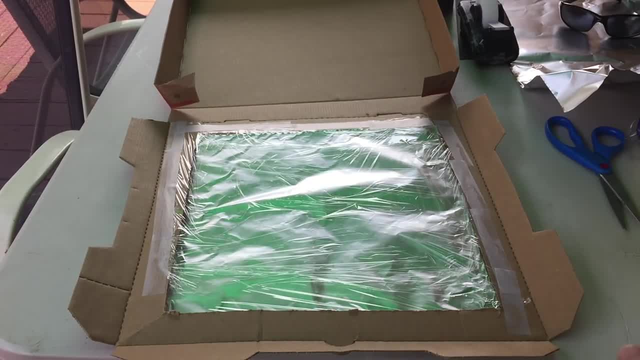 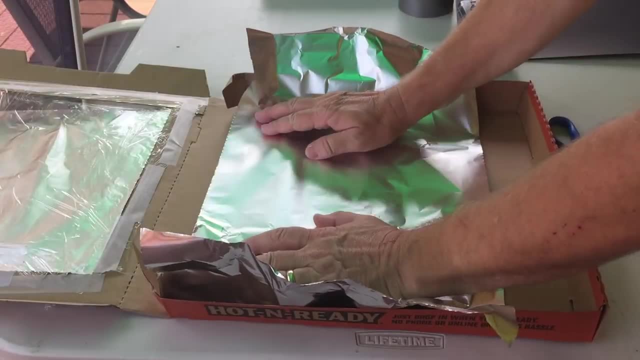 really quick, and then I added one more piece to complete the whole thing. So now I've got my plastic lid over the cutout portion. Now I'm going to layer the inside of the pizza box, so the foil is covering the whole bottom of the. 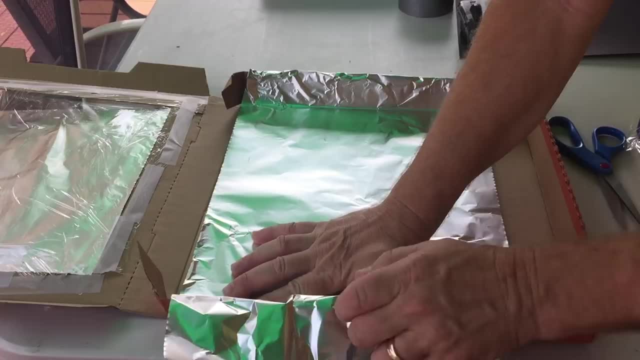 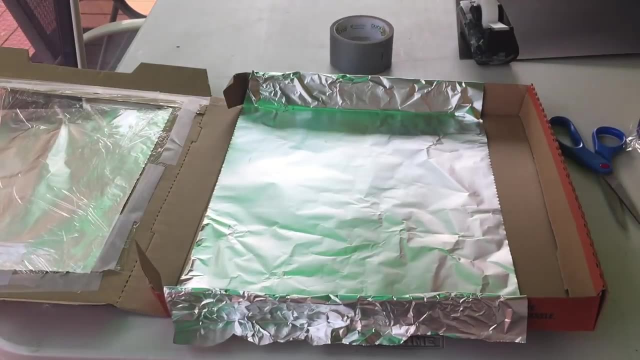 box. So you kind of just want it to fold over to the end, and then you're going to cut it out, and then you're going to cut the aluminum foil just about halfway to the side of the box so we can tape it down again. You really don't need to. 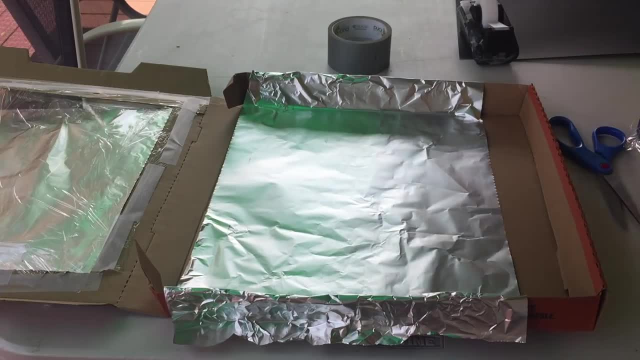 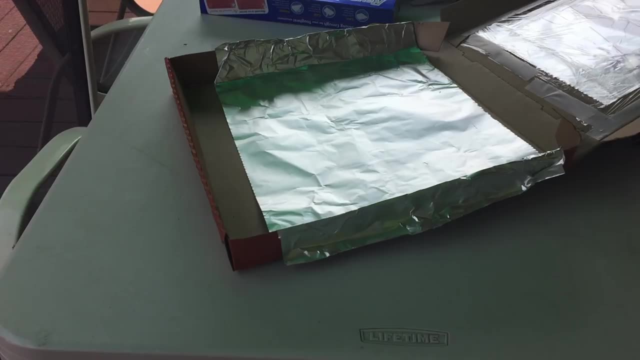 tape it. but I find after you move it around a little bit it is a little bit better if we tape it. So then you're going to also have a second piece right here that you're going to cover up the rest of it. So once we get the first piece, here I am. 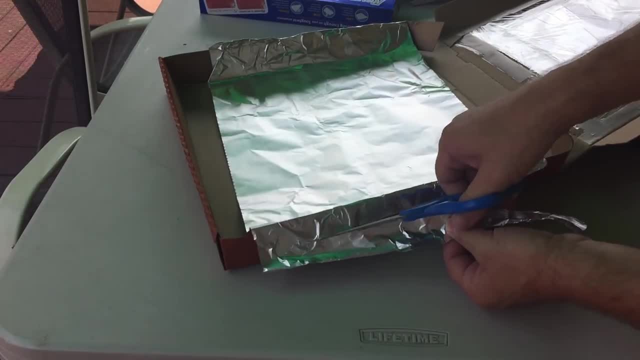 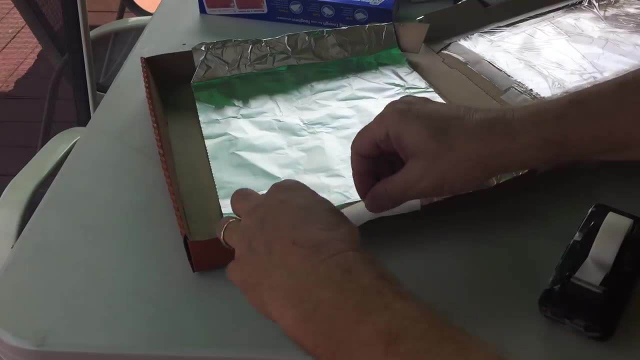 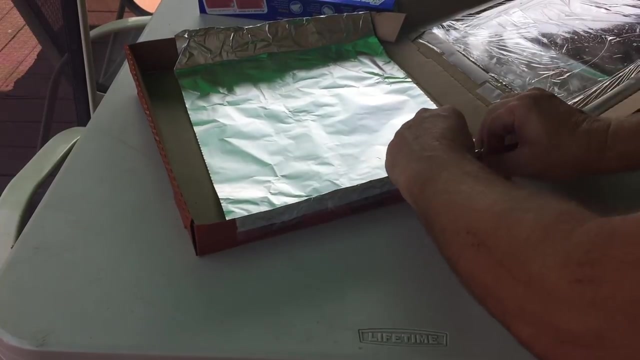 going to cut the foil, or you could actually just measure it right the first time- where I didn't measure it right the first time, And then you're just going to tape that piece Right here And you're going to do this on the same on both sides. So I will speed it up and we'll get this done. So I'm doing this. 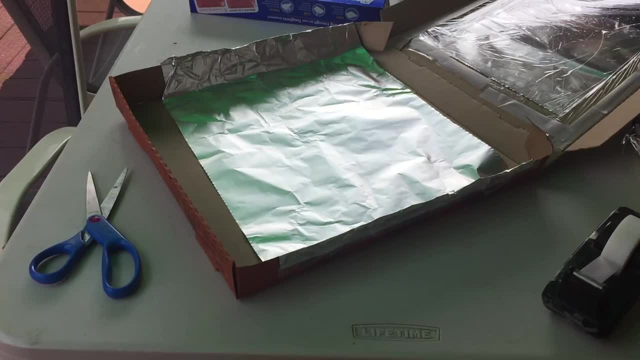 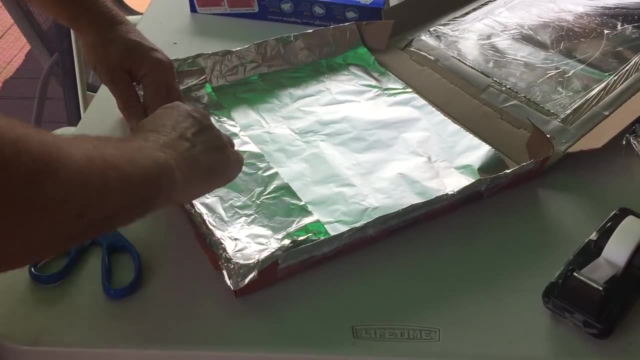 side right here. I got it in fast forward so it's going quick. I'm going to put I cut the piece this time as being smart and learning from my mistakes the first time. I cut it in so it fit in just right. I don't use any tape on the inside, but I'm going to 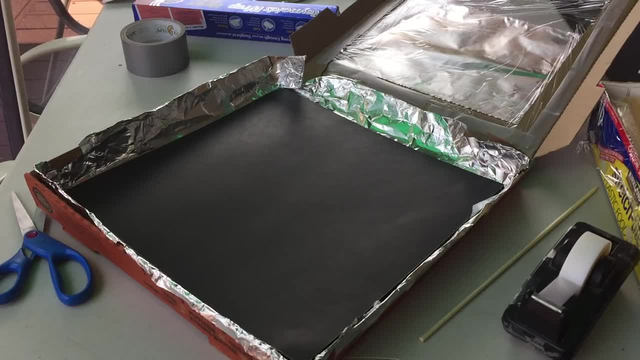 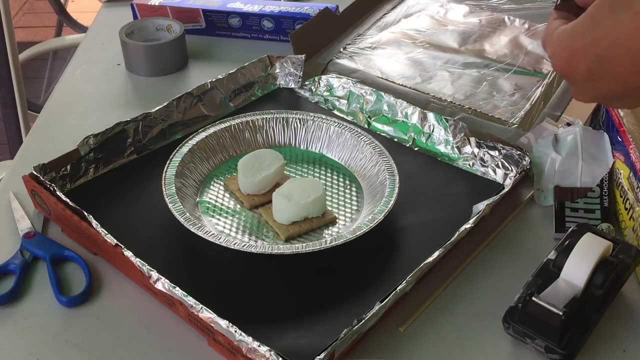 tape the outsides of them so it holds down. Then you're going to cut out a piece of black paper, put it on the bottom of the pan. Then I just took a regular pie tin and put my s'mores. Now the recipe's a little bit different here, Instead of putting the 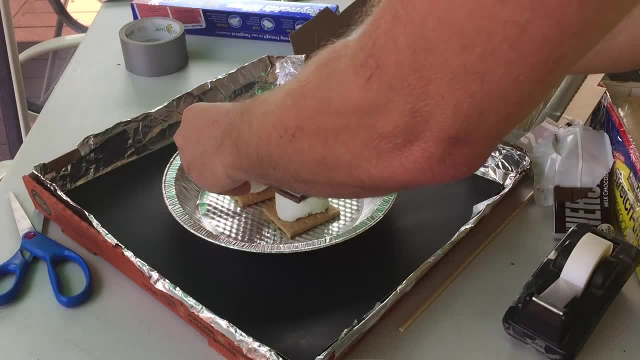 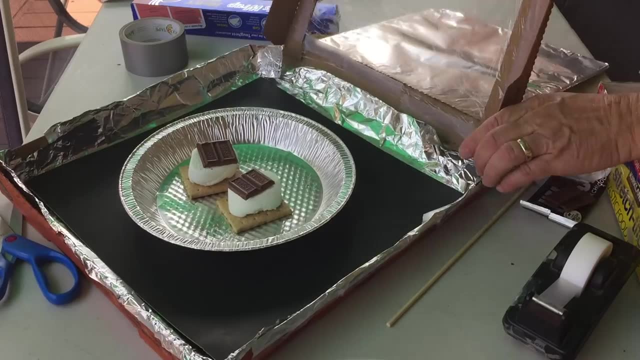 chocolate, the graham cracker chocolate, the marshmallow. when you use a solar oven, I find it better if you use the graham cracker marshmallow chocolate, because the marshmallow you need to cook a little longer. So it works better this way, But you can try it both. 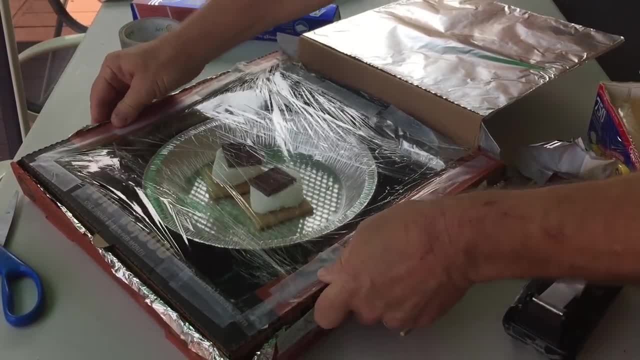 ways, Then you're just going to close the pizza box. And if you feel like it's not going to fit, you're going to close the pizza box. and if you feel like it's not going to fit, you're going to close the pizza box. And if you feel like it's not going to fit, you're going to. 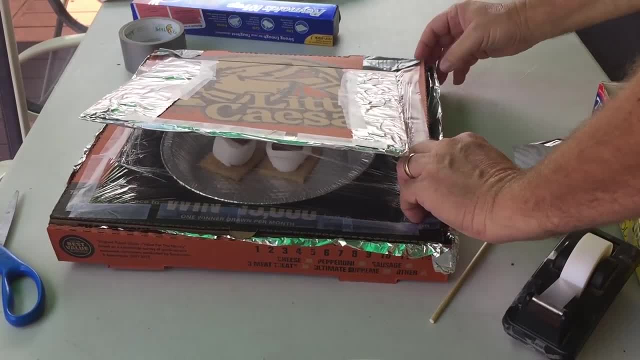 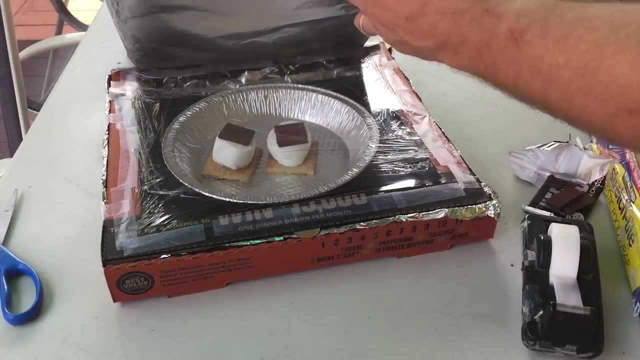 close it all the way. You can tape the sides on temporarily. Like you can see, mine's not really holding there, So I'm going to end up taping those sides down. And then, now I've got those sides taped, You take your skewer and you put it in. There's little holes on the side of the pizza box. 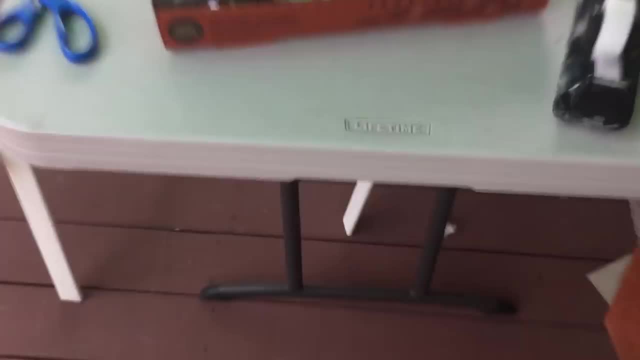 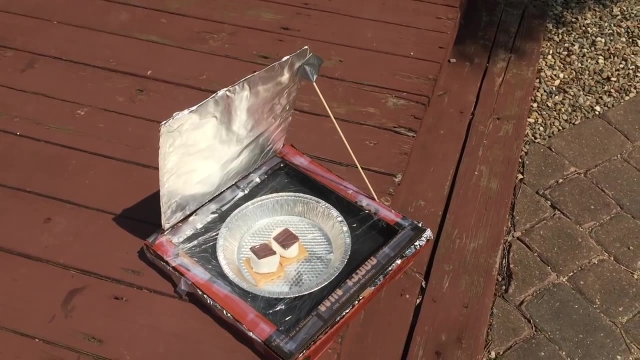 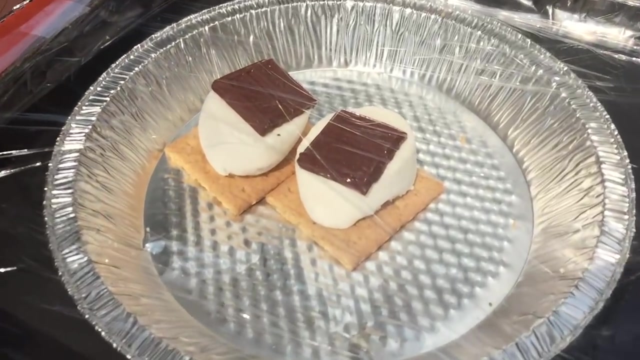 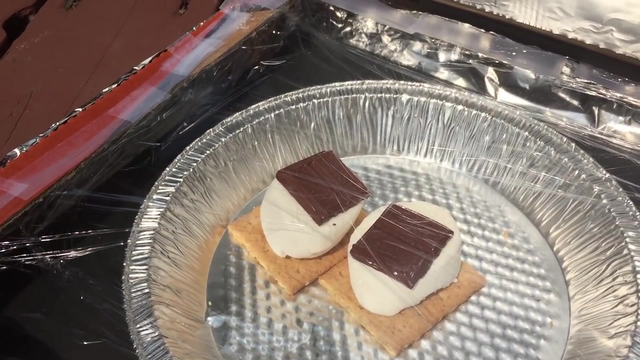 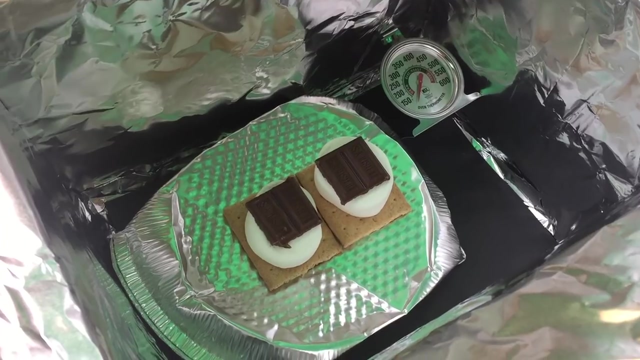 Prop it up against the little lid we have there And we're going to tape that in once we get into the sun. You want it to angle the exact angle so you can see there's enough reflection coming down. So therefore, the ones that are 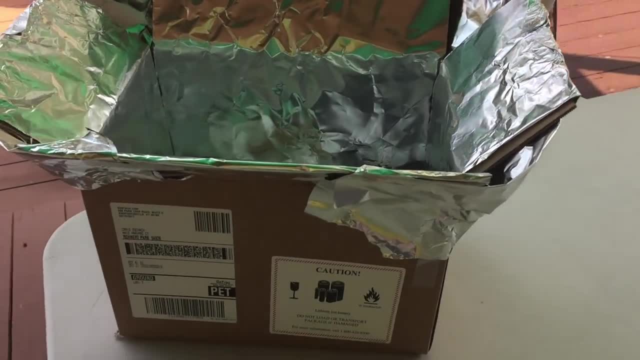 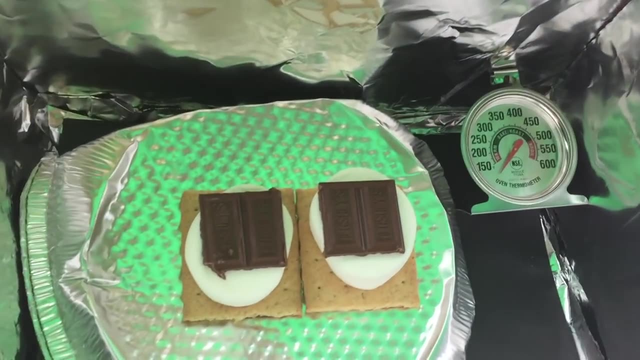 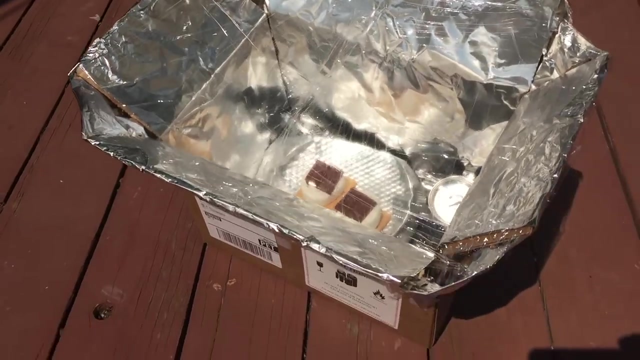 and then I put a little corner edges around so it kind of goes all the way around. that's optional tape down all the outside of the foil, no tape on the inside, and then I put black on the bottom and then a pie pan I tipped upside down. I also put a thermometer in there so we can see the 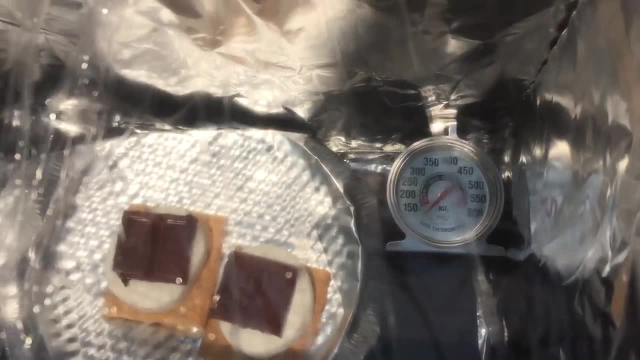 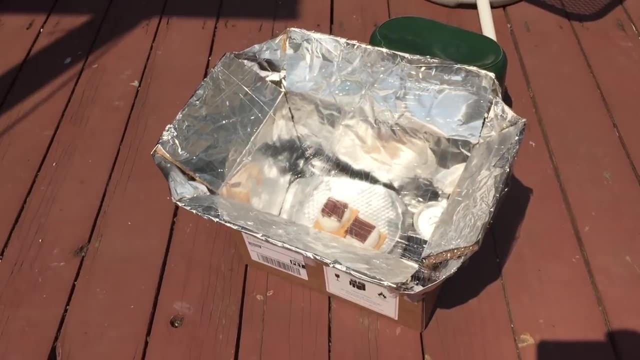 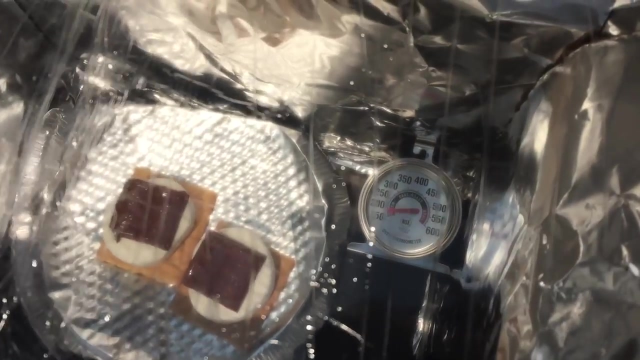 temperature this time, and then I covered it completely with with saran wrap and taped it, so it's completely sealed in and I believe this is going to cook a lot faster because it has more area of of aluminum. so I've got two different uh solar ovens going at the same time. um, we started. 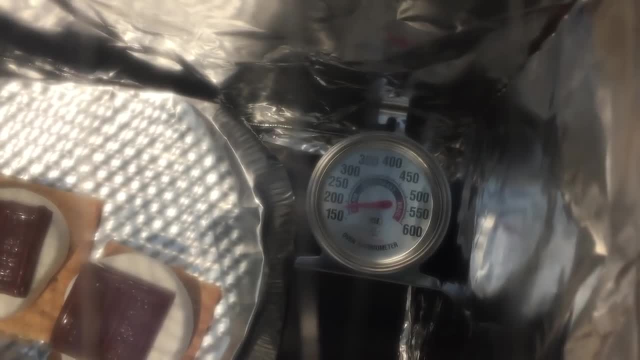 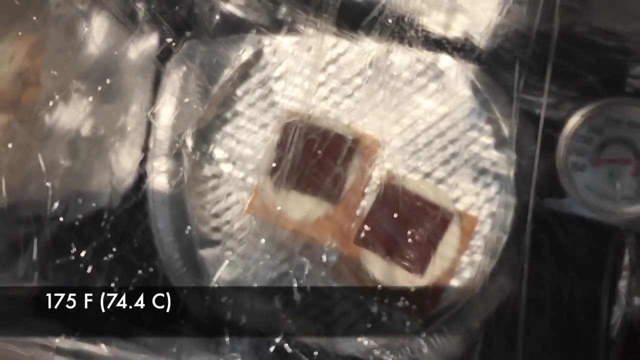 off at zero. it's already at over 150 degrees inside that box, so we'll see where it gets to. so while I'm waiting for my snack to be done, I'm going to explain, uh, the science behind this. so the solar cooking is done by the means of the sun's uv rays. it is not the sun's heat that cooks. 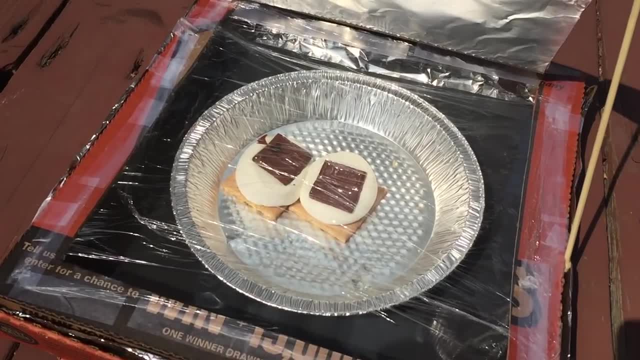 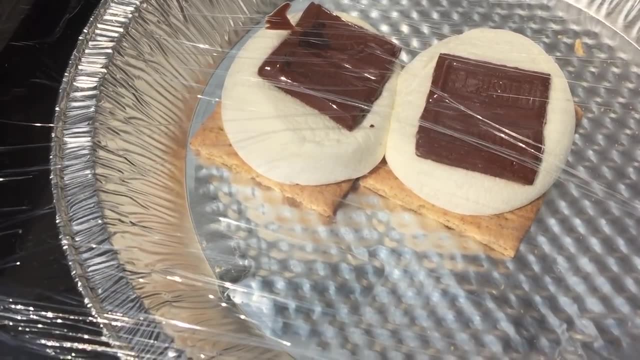 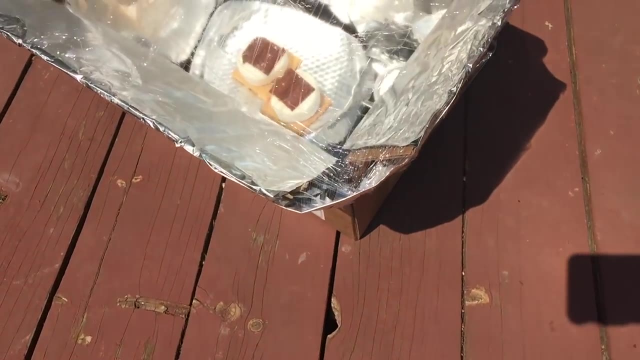 the food. nor is the outside uh temperature, though this can somewhat affect the rate of the time required to cook, as today being very hot, but rather it's the sun's rays that are converted into heat energy that cooks the s'mores or other food. so the heat of the sun is trapped inside the box or the pizza box and it starts getting very hot. 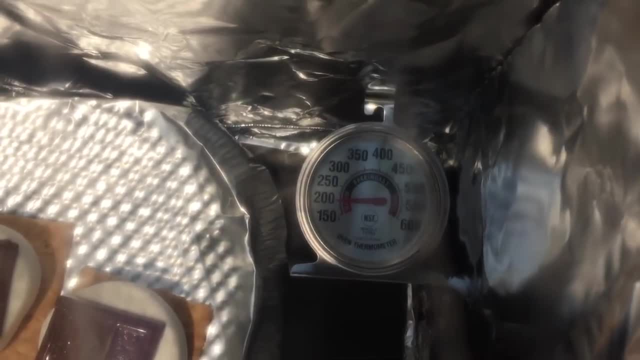 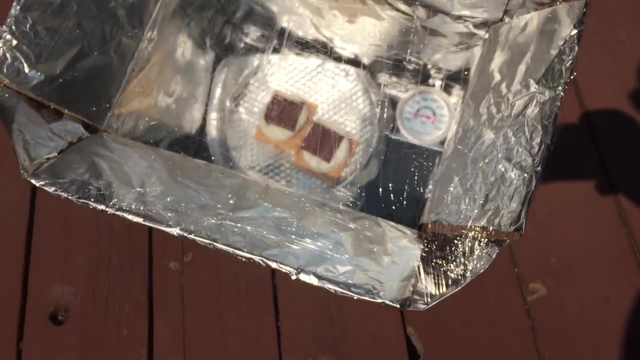 ovens like this are also called collector boxes, because they collect the sunshine inside as it sits out in the sun. our oven eventually heat up enough to melt cheese or or even cook a hot dog, or like a hot dog or something like that, so it's going to cook the sun's rays that are converted. 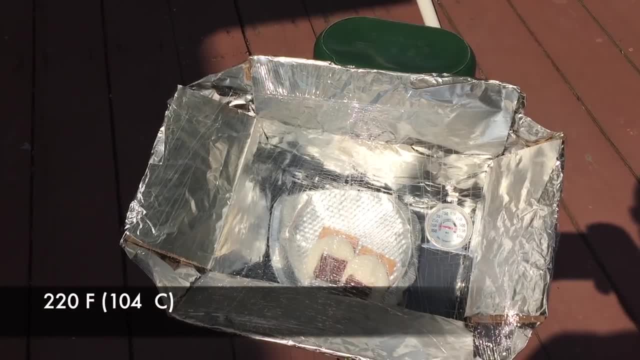 into heat energy that cooks the s'mores or other food. so the heat of the sun is trapped inside the s'mores, like we're doing. how does this all happen? well, the rays of the light are coming to the earth at an angle. the foil reflects those rays and bounces them directly into the open box once. 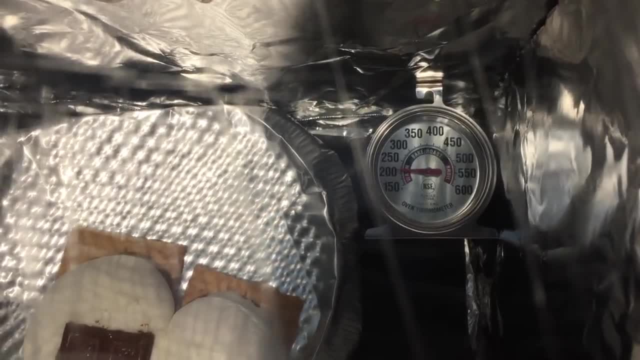 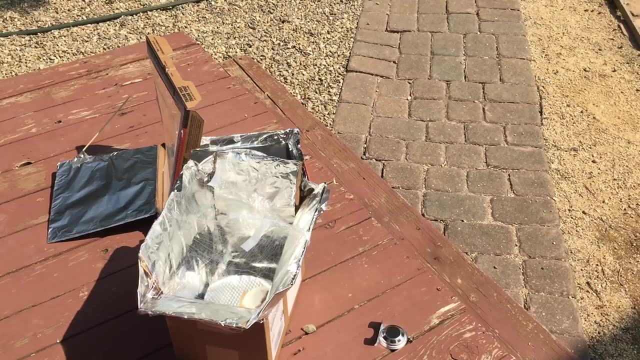 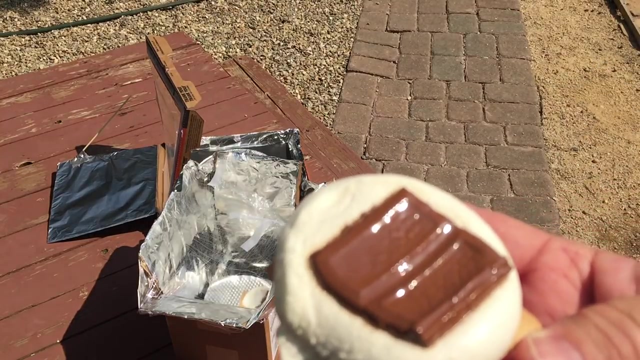 it's gone through the plastic wrap. it heats up the air that is trapped inside. remember we sealed the plastic saran wrap. the black paper absorbs the heat on the bottom of the oven. so solar ovens can reach up to about 200 degrees fahrenheit, which today we got up to 225 on a sunny day and it 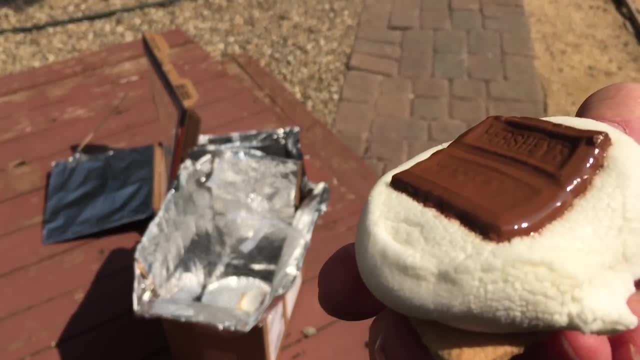 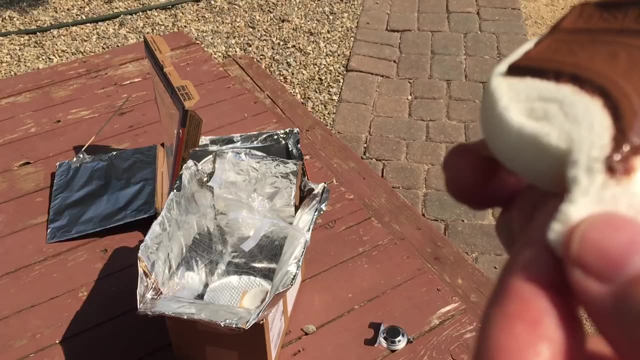 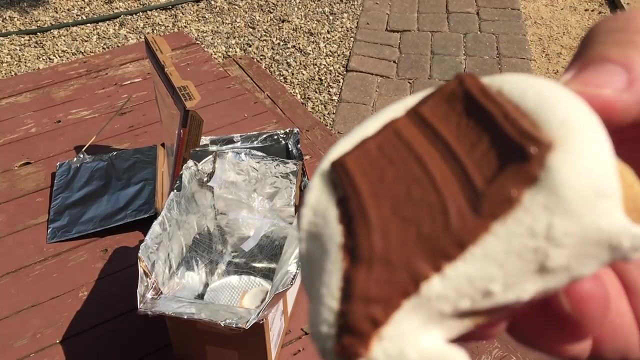 can take a lot longer to heat things in a conventional oven. although this method will take longer, it is very useful and easy and it is safe to leave alone while your energy from the sun cooks your food. this is a s'more from the pizza box oven- solar oven- and you can see the marshmallow.